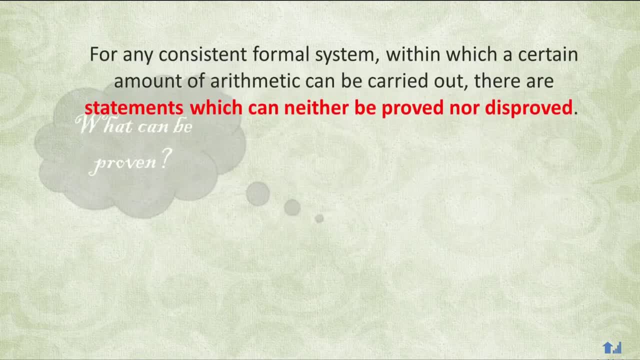 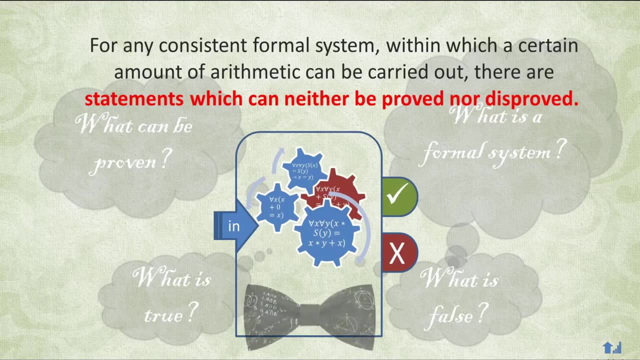 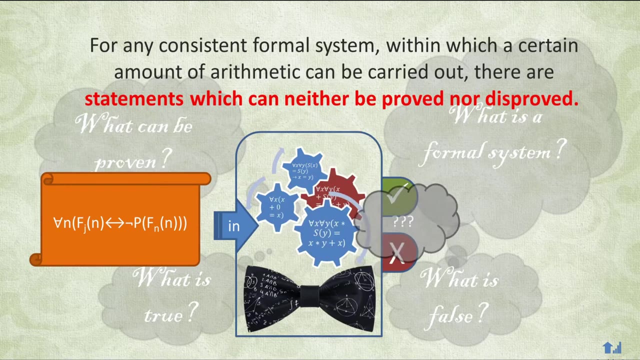 Gödel's incompleteness theorem states that, for any consistent formal system, there are statements which can neither be proved nor disproved, thereby setting bounds to what mathematics could prove. While it took Gödel's unmatched genius to show this, is there a simple explanation of how the 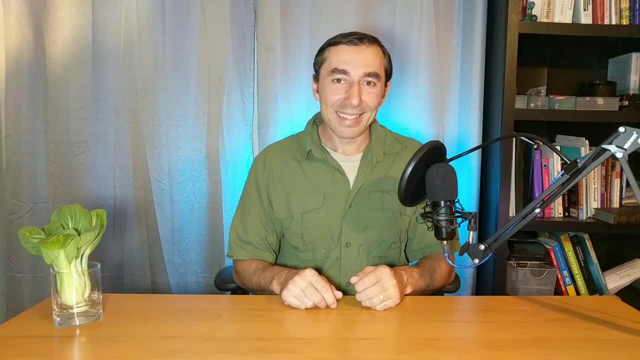 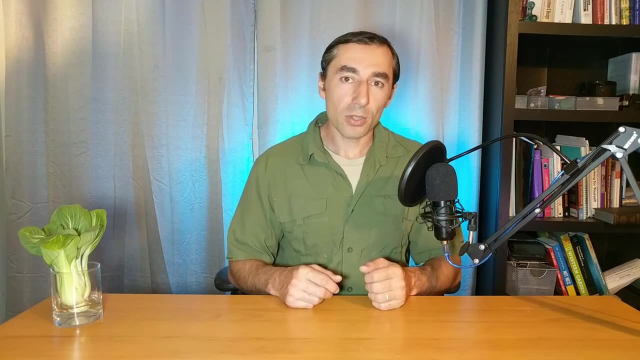 theorem was proved that the rest of us mortals could understand. Hello and welcome to Stablesort. In this episode, we're going to examine the context for the theorem in order to get a gist of what it's all about, and then we'll step through a semi-formal proof of it for those who'd like to dig a little deeper. 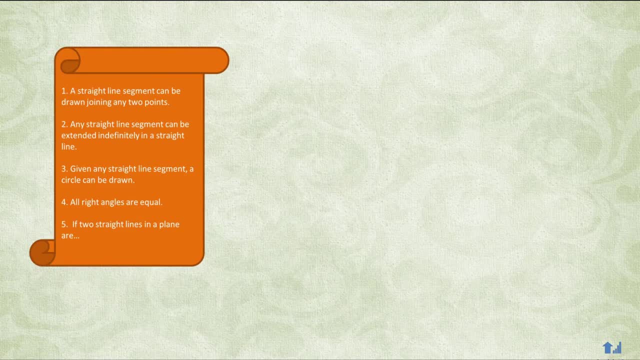 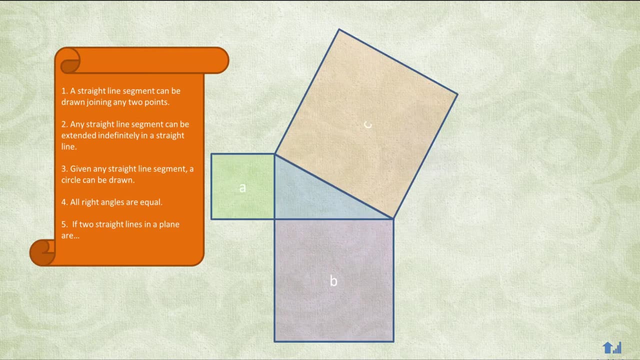 Let's first take a moment and recall how Euclidean geometry is based on a small set of axioms. Using these axioms, you can then derive all other theorems of Euclidean geometry. Mathematicians have strived to axiomatize their own branches of mathematics. 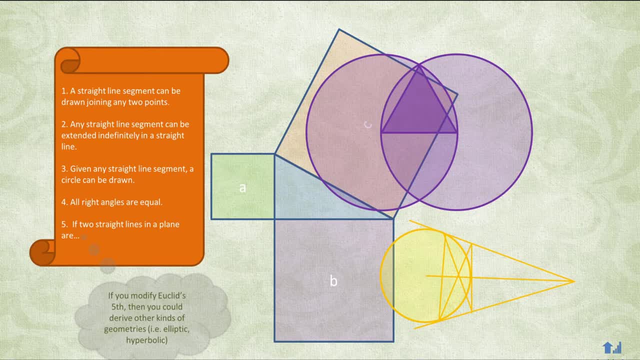 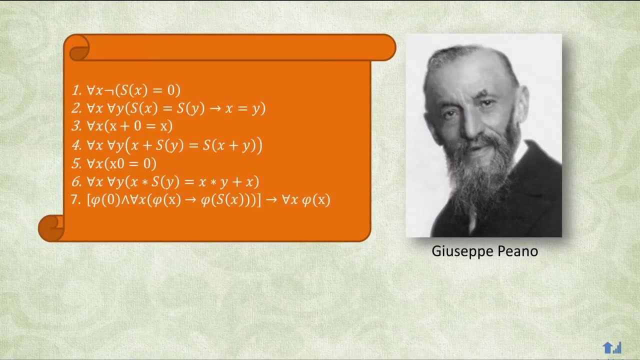 with the smallest set of axioms, that would still allow them to derive the largest set of theorems. One such mathematician was Giuseppe Piano, who formulated axioms for arithmetic of natural numbers. Natural numbers are the simplest ones. They are the non-negative integers 0,, 1,, 2,, 3, and so on. 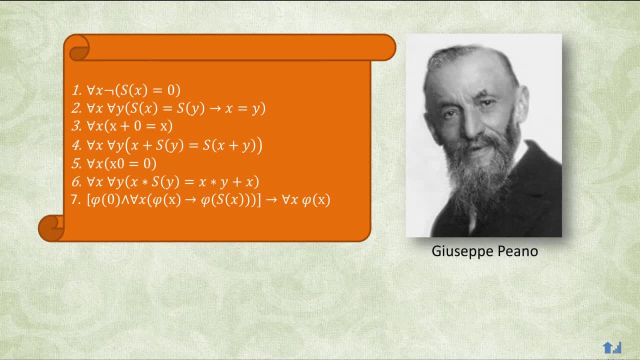 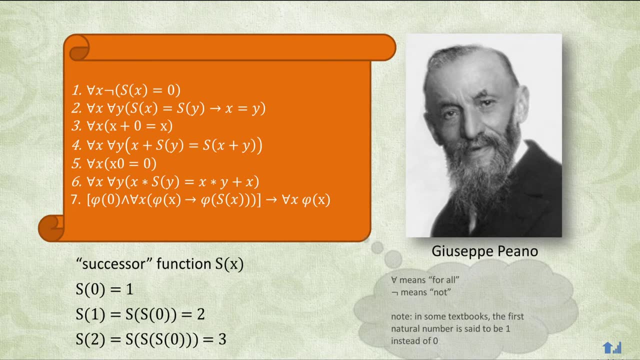 The value 0 is defined axiomatically as the first natural number, Then the next and all following natural numbers are defined by a successor function. The nice thing about this definition of natural numbers is that we get an intuitive sense that these numbers could be used for counting. 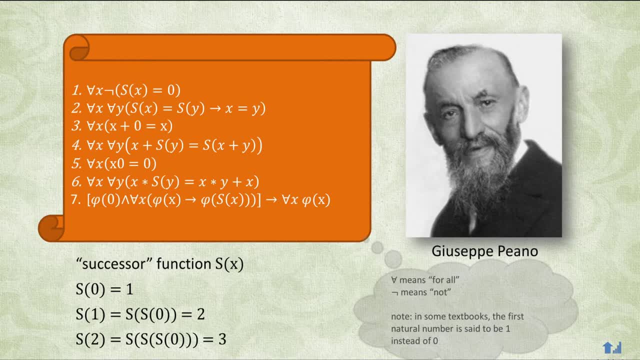 Given a natural number, you can always get the next natural number. In contrast, you could never have a successor function for real numbers, since real numbers are in a continuum and there is no such concept as the next real number. This is important because counting theorems or otherwise enumerating theorems, 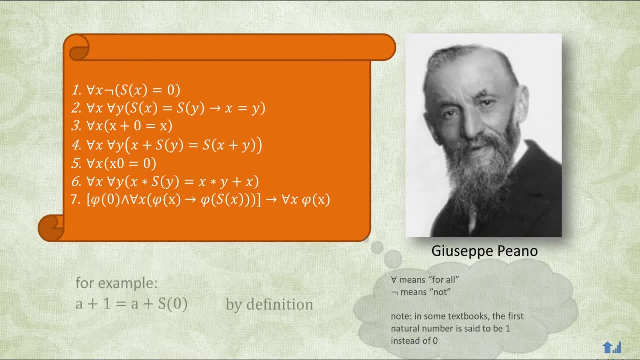 is at the heart of Gödel's argument. Based on these axioms, Piano formulated the arithmetics of addition and subtraction. Based on these axioms, Piano formulated the arithmetics of addition and subtraction. Based on these axioms, Piano formulated the arithmetics of addition and subtraction. 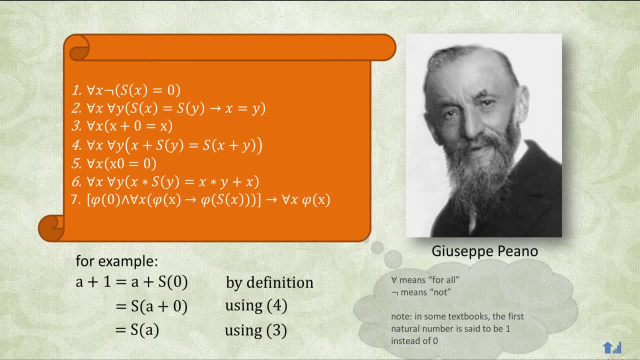 Which are the basis of other theories of natural numbers. A collection of this type of formulations is called a formal system. The axioms themselves are assumed to be true, while theories stated in a formal system can be derived if one is able to construct a sequence of logical operations. 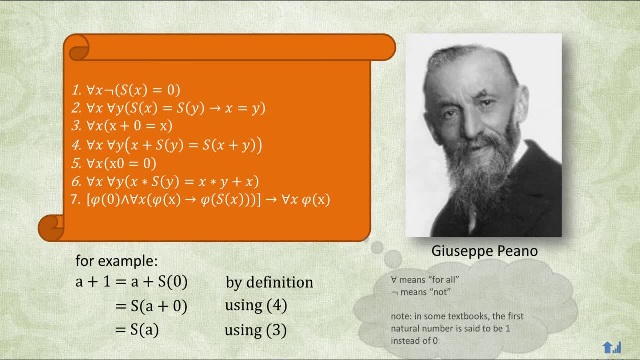 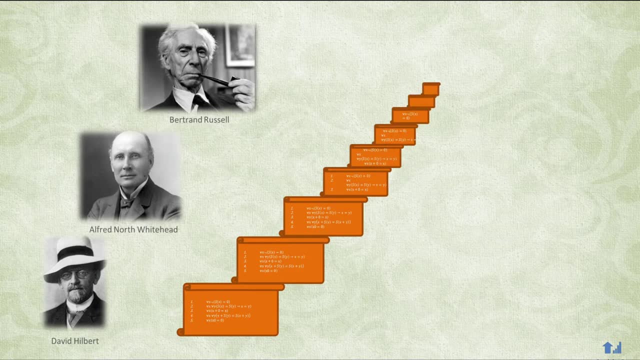 based on the axioms and the rules of axiomatic inference. At the start of 20th century, mathematicians had a sense that, given just the right set of axioms of a formal system, any mathematical theory could be proven to be true or false. 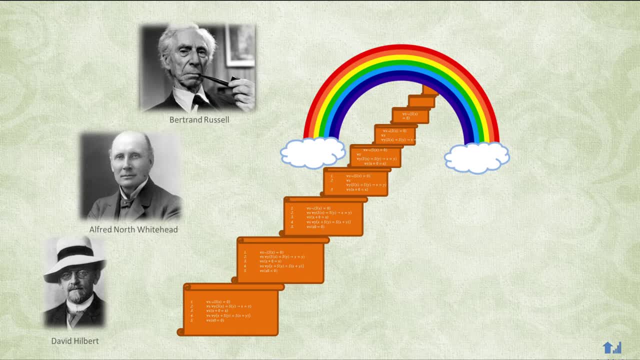 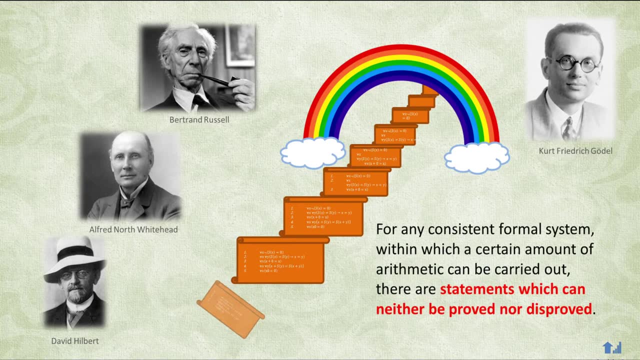 by systematically applying these axioms in the chain of logical operations. This is where Kurt Gödel, in his 1931 paper, shook the foundations of mathematics, proving that for any consistent formal system within which a certain amount of arithmetic can be carried out, 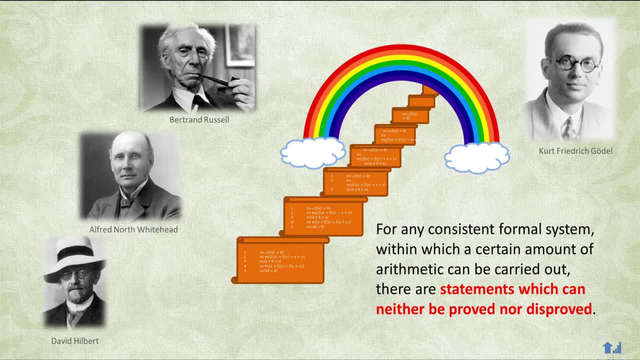 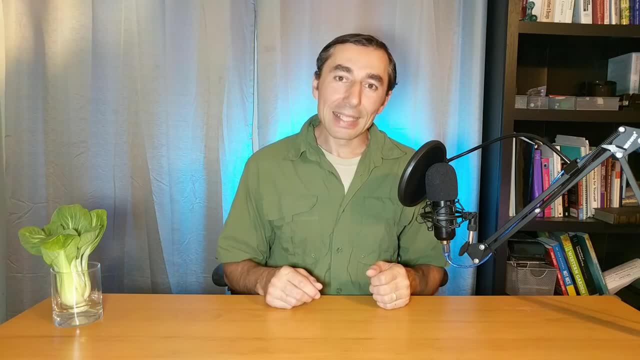 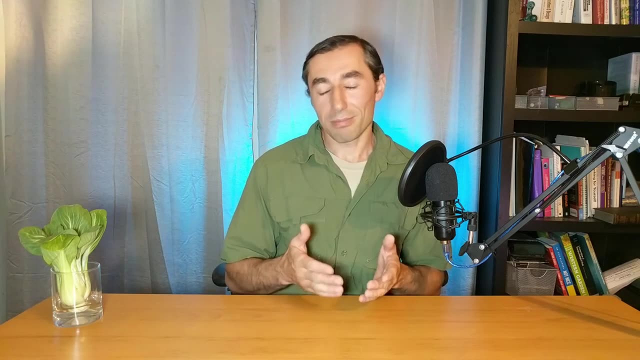 such as piano arithmetic. there are statements which can neither be proved nor disproved. Now that we have a sense of what axiomatic systems are, let's dispel the myth that the theorem applies to any kind of statements. For example, the statements God exists or, if you prefer, God does not exist, may have no proof. 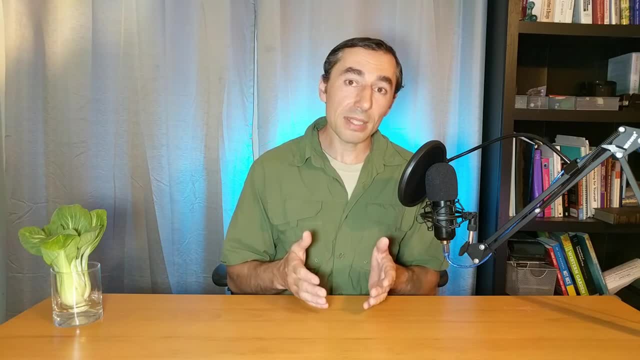 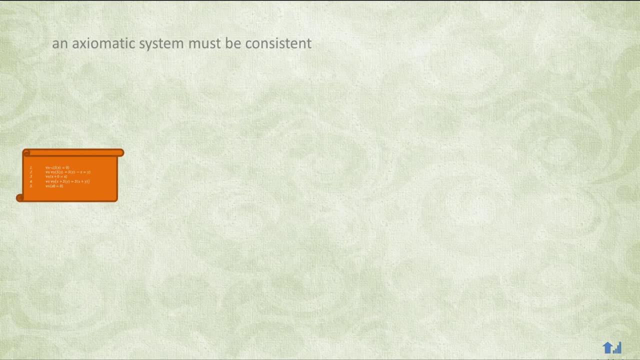 but the theorem does not apply here at all, since those are statements in English language, which is not axiomatic. The theorem applies only to axiomatic systems. Moreover, the axiomatic system must be consistent, which means that no statement and its 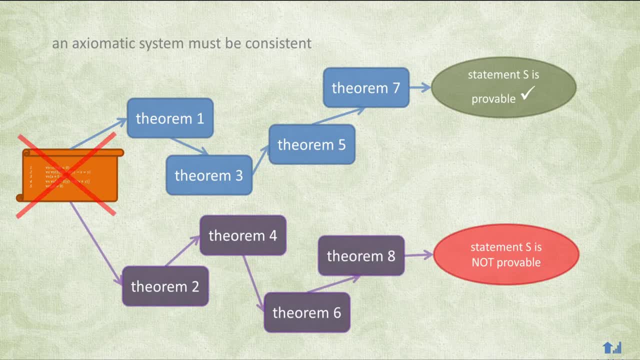 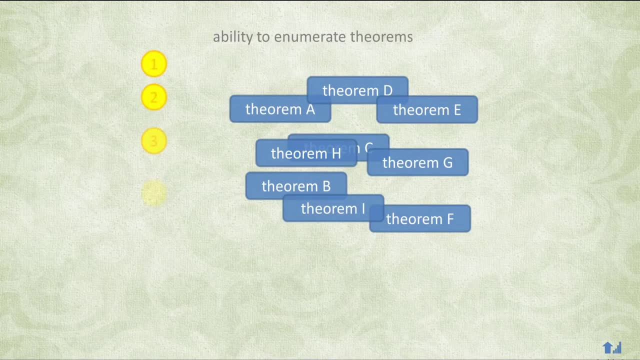 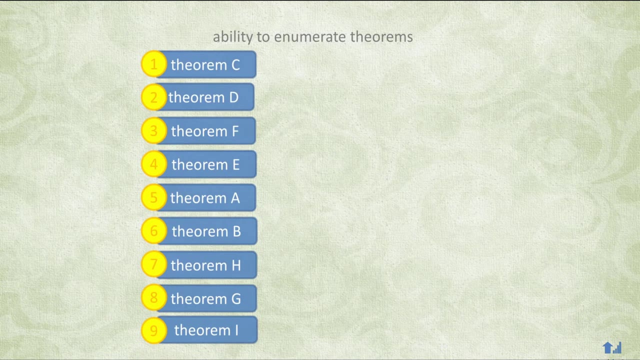 negation can both be derived by just following a different sequence of axioms and theorems. And finally, the mention of certain amount of arithmetic refers to being able to at least enumerate the theorems of the language. So a very simple system that has no computing power. 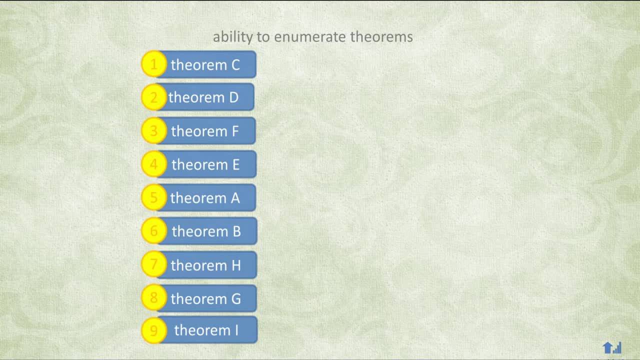 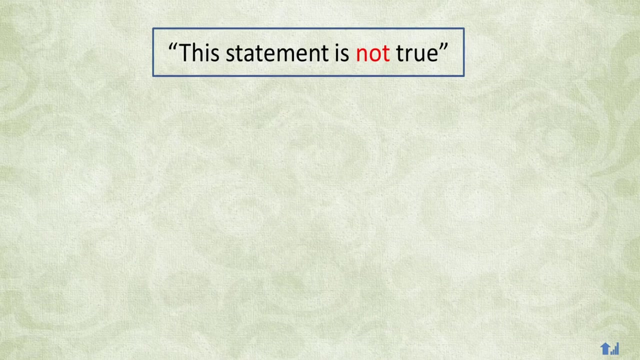 may in fact be consistent and entirely complete, But then it also won't have the power needed to express even simple computations. Let's now examine how Gödel proved his theorem. In essence, he constructed a legitimate, well-formulated mathematical statement that implied that 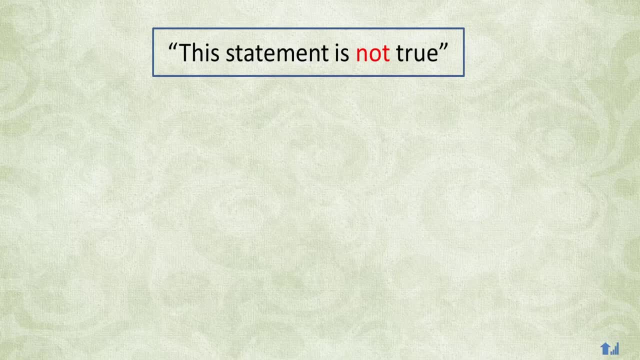 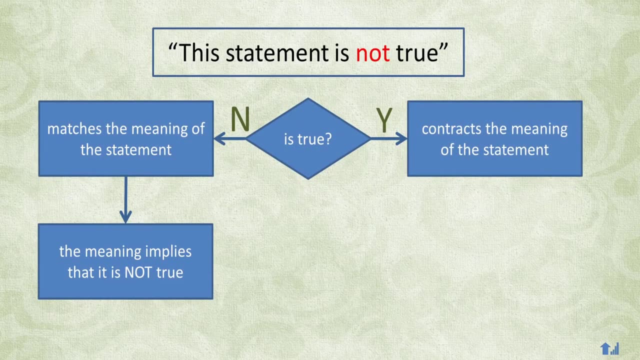 it itself is not provable. To construct such a statement, we start with this linguistic paradox. This statement is not true. Simply reading it out presents a problem, since if we were to assume that the statement is true, its meaning would suggest the opposite. 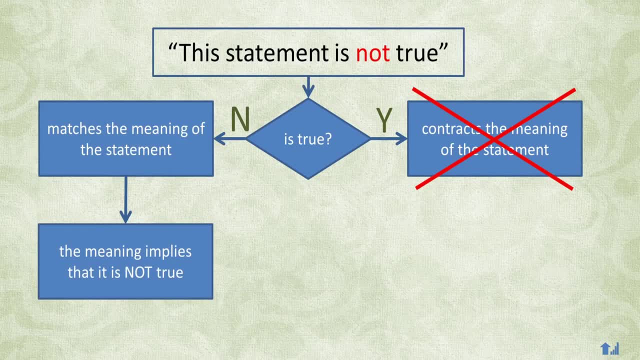 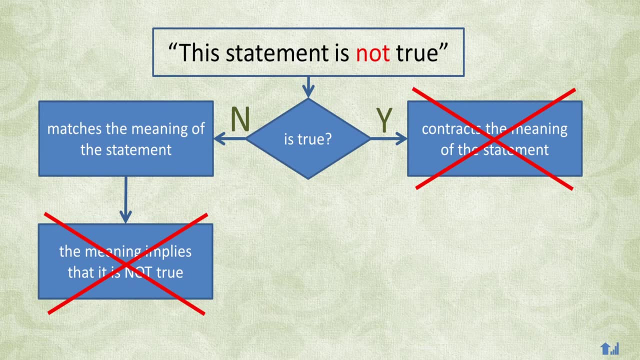 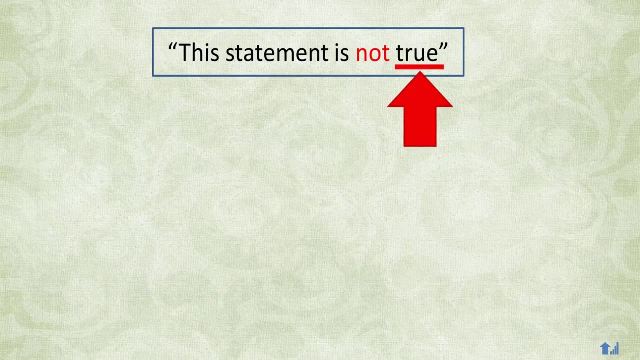 On the other hand, if the statement is not true, then its implied meaning turns out to be true. hence the paradox. So what would it take to construct a similar statement but express it formally? in mathematical notation, There are two immediate problems to handle. First of all, the word true. somewhat surprisingly, 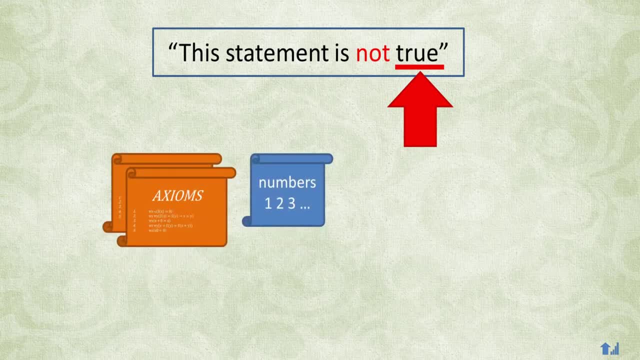 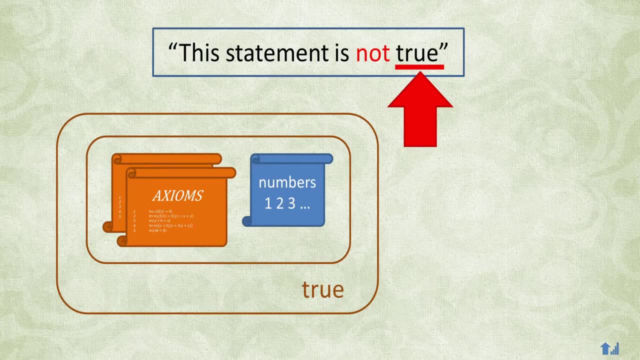 is not defined axiomatically. Numbers and formulas don't have a property of true. We think of axioms as being defined to be true, and any theorems that are derived from them would therefore also be true, But the concept of truth would then still be. 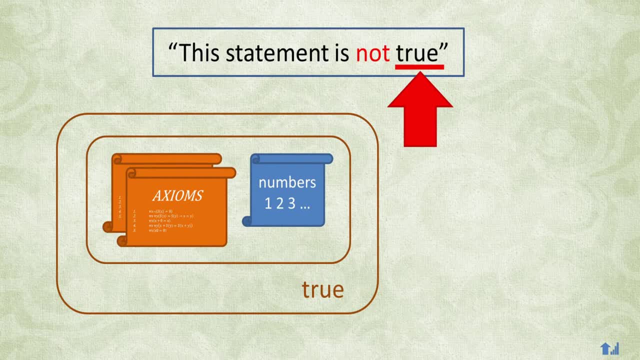 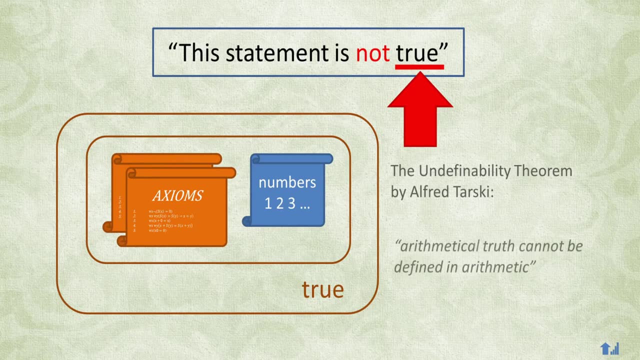 defined as true. The problem is that truth is not defined in the same way as the system itself. This is a very nuanced subject and it's worth more investigation in its own right. For more on this, check out the Undefinability theorem by Alfred Tarski, which roughly states: 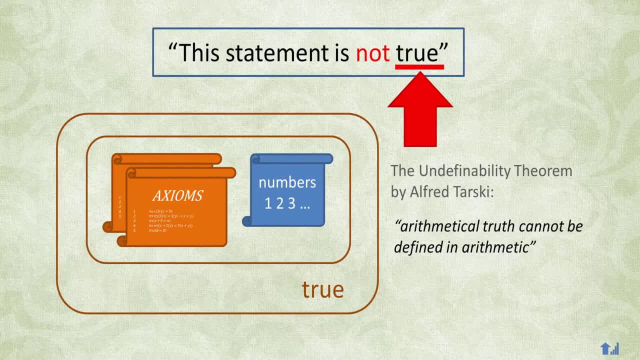 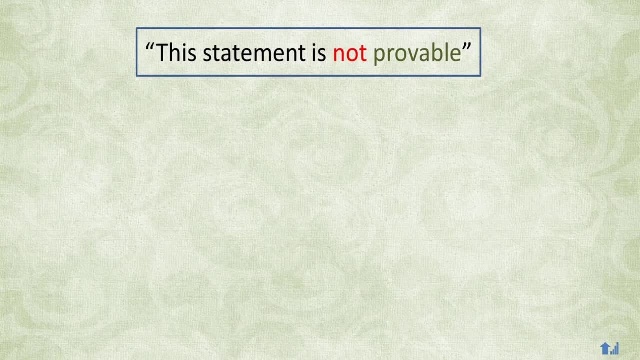 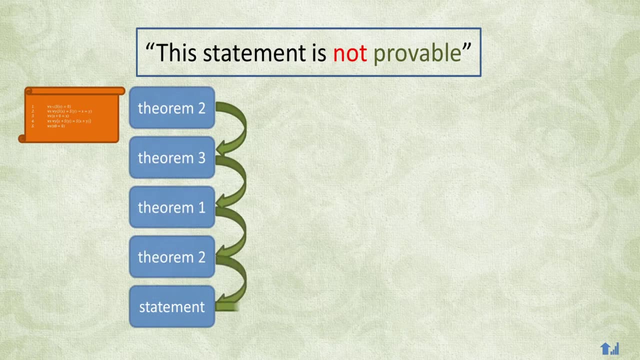 that arithmetical truth cannot be defined in arithmetic. It's linked in the description, But Gödel avoided this issue by instead relying on the word provable, which does have a specific meaning. So you could have a computer program that takes in a statement. 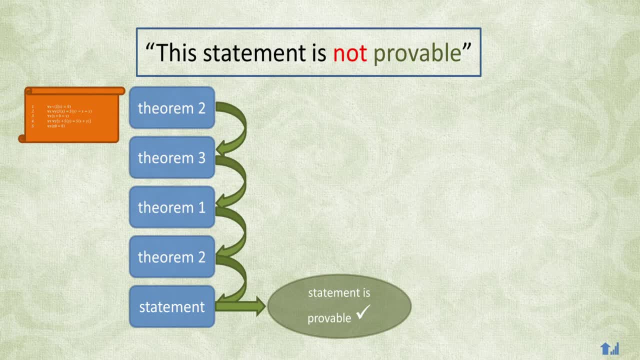 as well as a proof of that statement, and decides in a purely mechanical kind of a way: if the proof is valid As in, it follows each line of the proof using the rules of axiomatic inference, If it reaches the last line of the proof and it matches the statement in question. 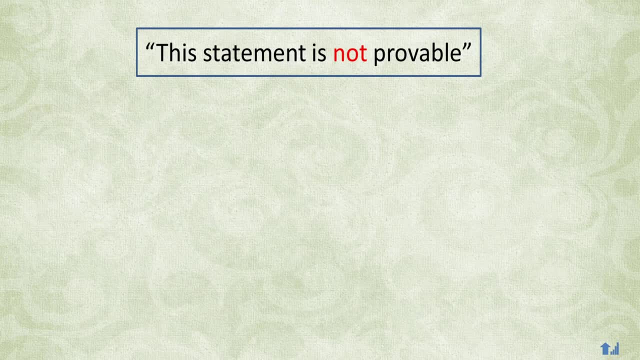 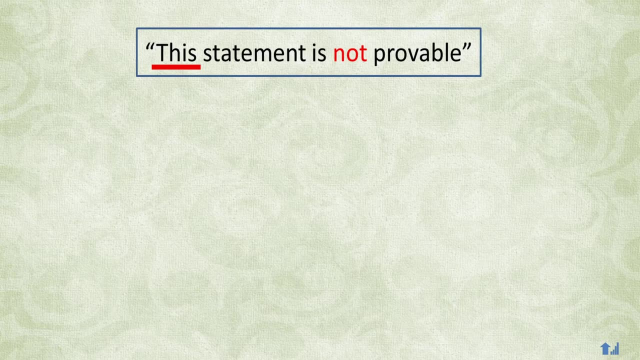 then the proof must be valid. The other problematic word is this: It refers to the statement itself without the statement having been defined yet. It's like saying this video is exactly 16 minutes and 9 seconds long without first having made the video. 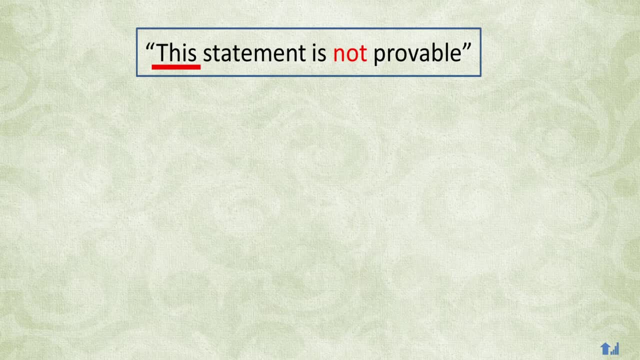 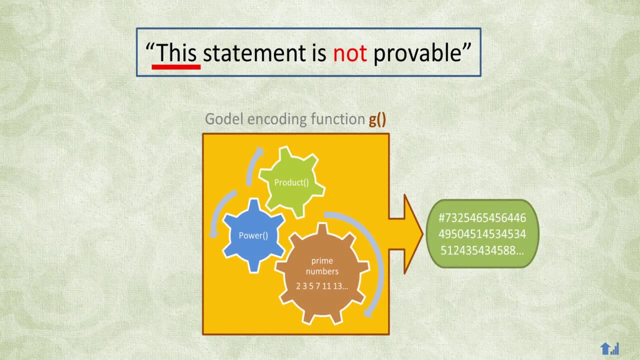 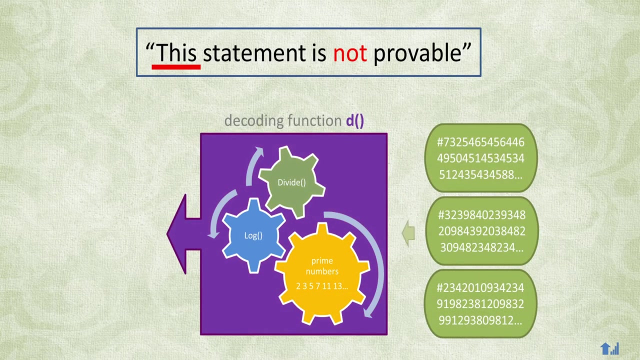 To get around this problem, Gödel established a way to convert statements such as theorems, and even proofs of those theorems, into natural numbers, as a type of encoding. Then, having listed encodings of specific kinds of formulas, he showed that there is a natural number in that list. 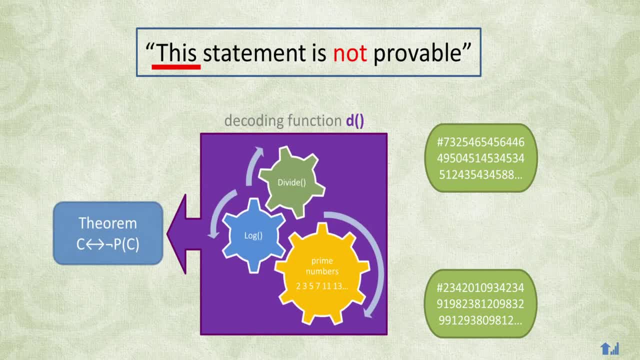 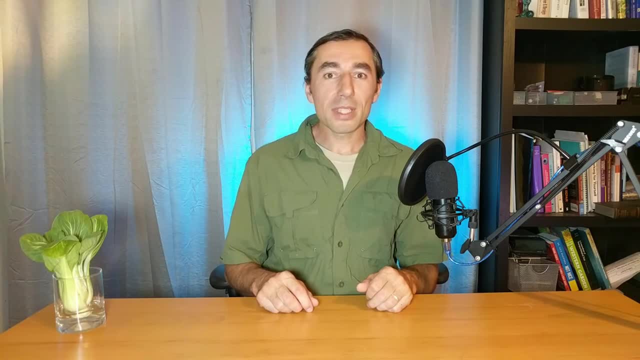 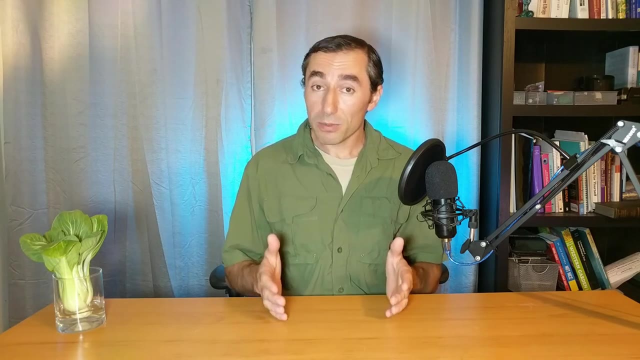 that corresponds to a formula that states its own un-probability. Perhaps at some point I'll make another video commenting on Gödel's original proof, But for today we're going to examine an abbreviated version of it, which is a lot easier to understand. By no means is it a formal proof, but still, hopefully it'll pave the way. 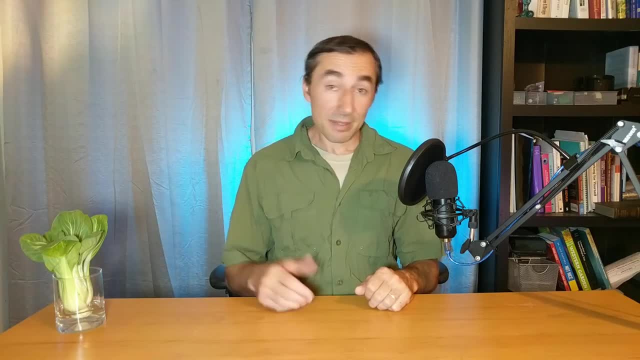 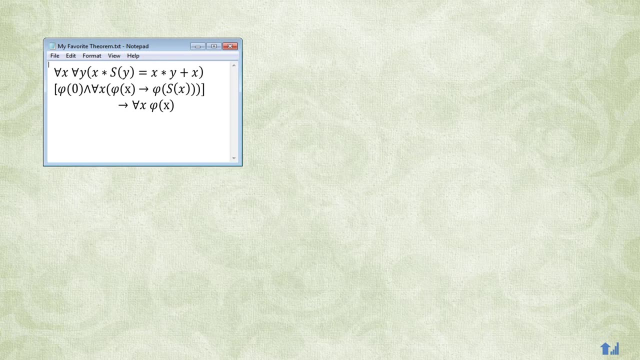 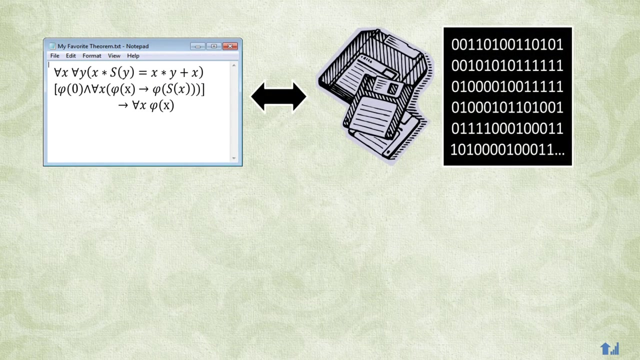 for you to read the original paper, English translation of which is linked in the description. Converting mathematical statements into a number is nothing special, After all. you can open a text editor type in some characters and then save that file. Those characters are converted into some encoding such as ASCII. 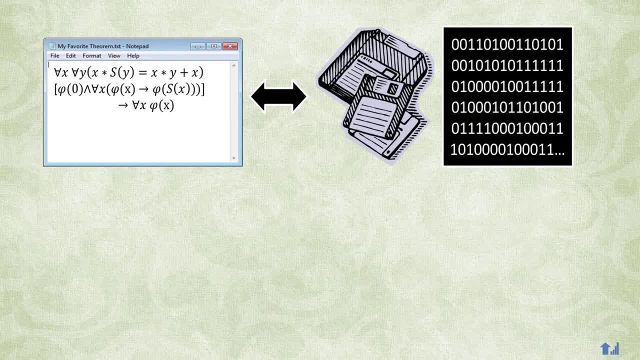 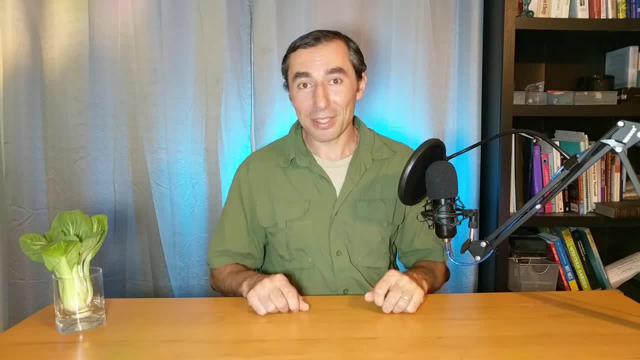 and then saved to disk and binary as a sequence of zeros and ones. So you can look at this sequence of zeros and ones as one huge number. At the time ASCII wasn't invented yet, Neither were programming languages, or even computers, for that matter. 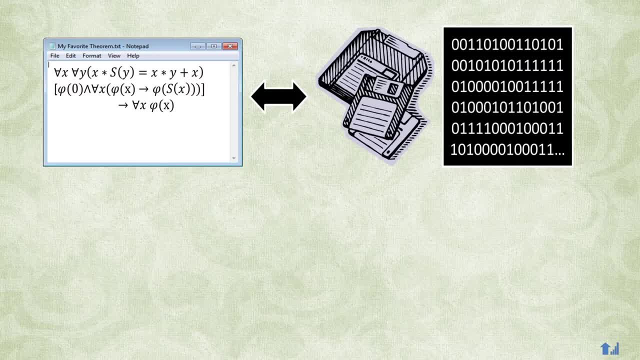 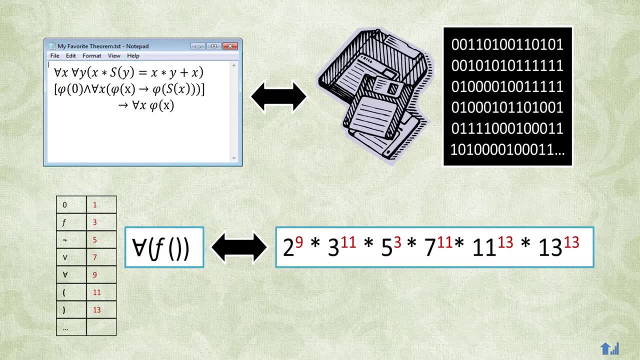 So Gödel resolved to doing it purely algebraically. His encoding involved assigning a unique number to each character, then taking the first n prime numbers, raising each of them to the power of the corresponding character and multiplying all of them into one giant number. This is called Gödel encoding. 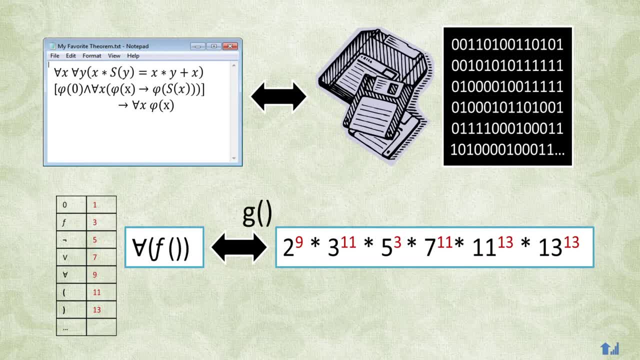 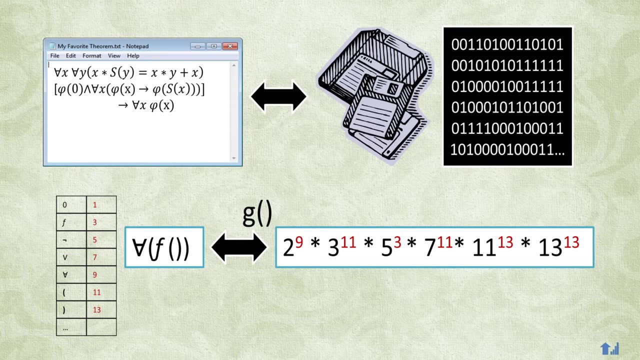 and could be represented by a function g. The point of all this is that you can convert that giant number back into the original sequence of characters by performing prime number factorization, which again is a purely algebraic calculation. The other point is that mathematicians for some reason love to make everything more. 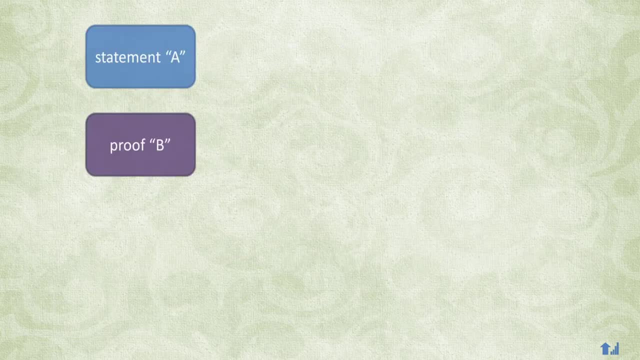 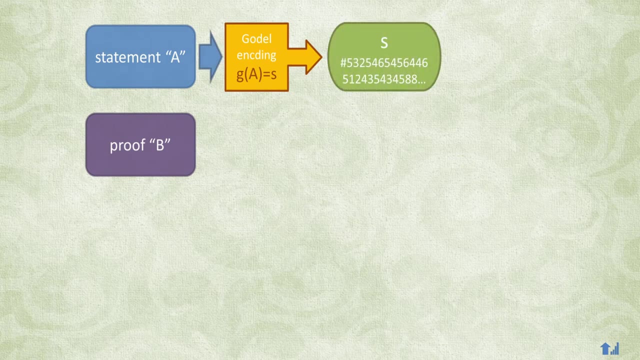 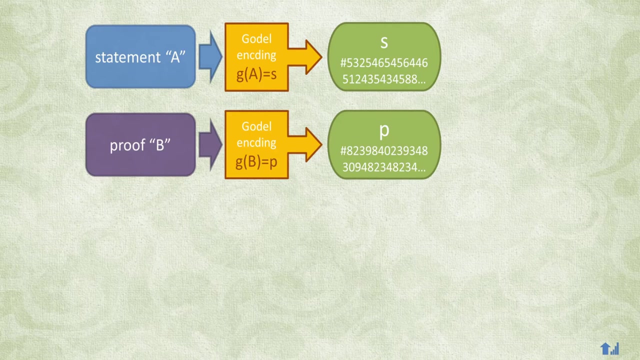 complicated than it needs to be. So Gödel encoding establishes a one-to-one correspondence between a unique sequence of characters and some unique number. This allowed Gödel to convert any mathematical statement, as well as a proof of that statement, into two unique numbers. Suppose we have 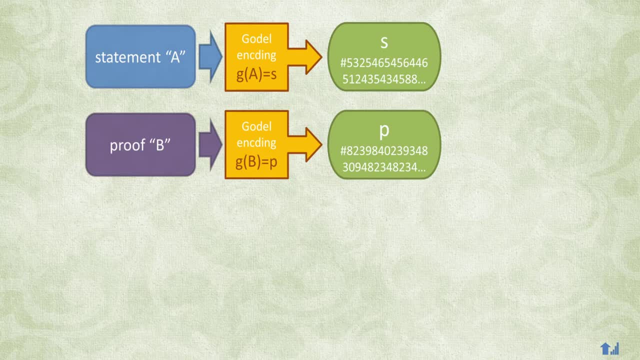 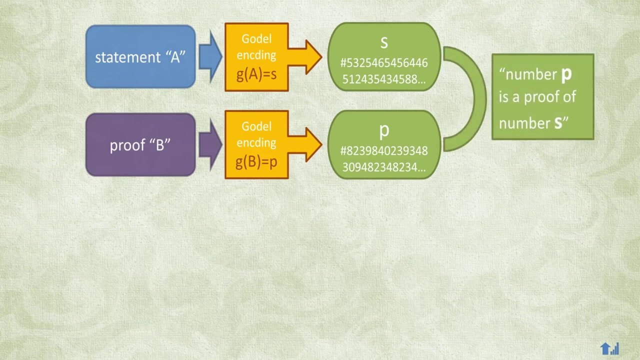 some statement A and a proof of that statement B. Using Gödel encoding function G, we encode both statements to get corresponding numbers S and P. The two numbers establish a specific kind of a relationship between the two. that could be read as number P is a proof of number S. 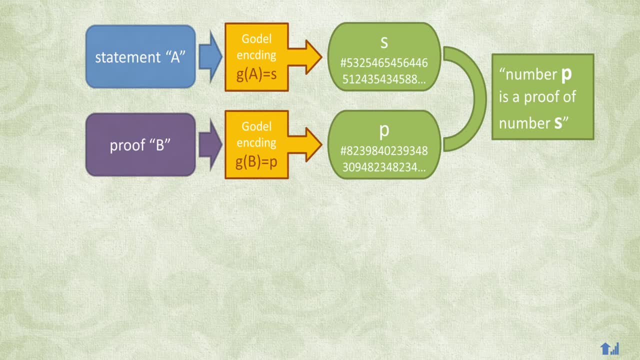 It's like a proof of number P. It's like a proof of number P saying 5 is a square root of 25, or 64 is a multiple of 32.. This is a purely mathematical property between the two numbers and therefore it could be checked purely mathematically. 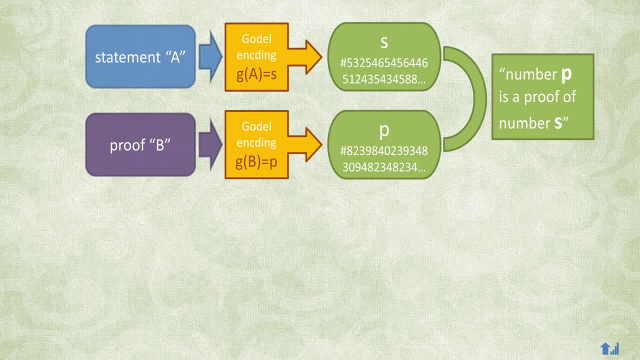 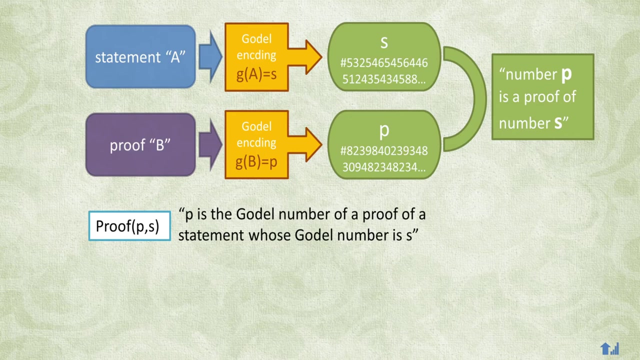 Much in the same way as you could have a function that checks if 64 is a multiple of 32, you could also have a function that checks if number p is a proof of number s. Let proof of p and s be a binary predicate. that translates: p is a Gödel number of a proof of a statement. 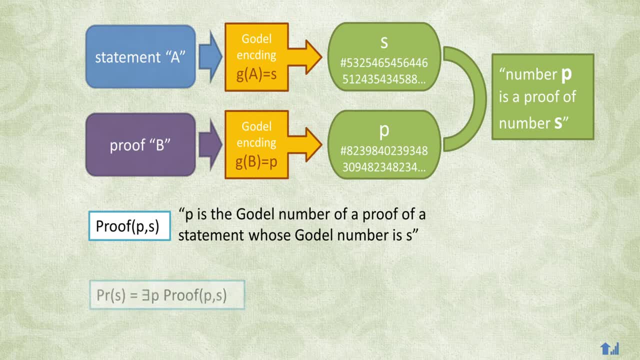 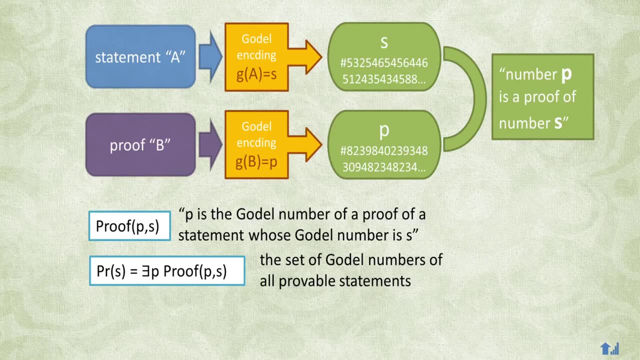 whose Gödel number is s. Then we define pr as the set of Gödel numbers of all provable statements. Since we can freely convert a statement into its Gödel encoding and then convert the Gödel encoding back into the original statement, we can further abbreviate. 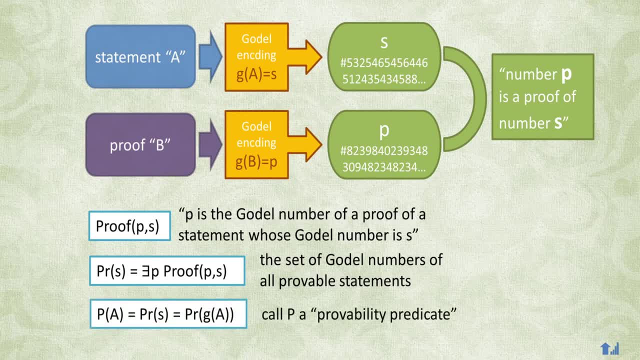 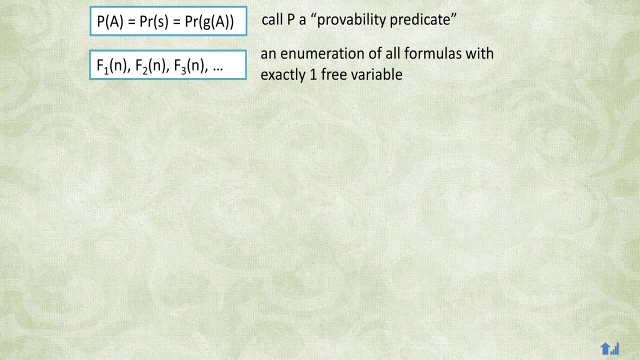 into p of a equal pr of s. pr of a is a provable predicate, and we can call p a provability predicate. Let f1, f2 and so on be an enumeration of all formulas with exactly one free variable. These are formulas of natural numbers. So for every natural number the functions produce. 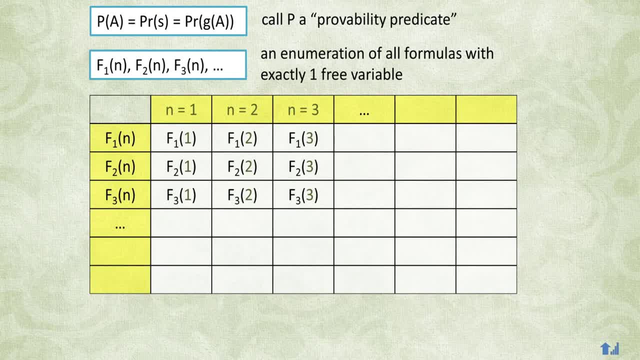 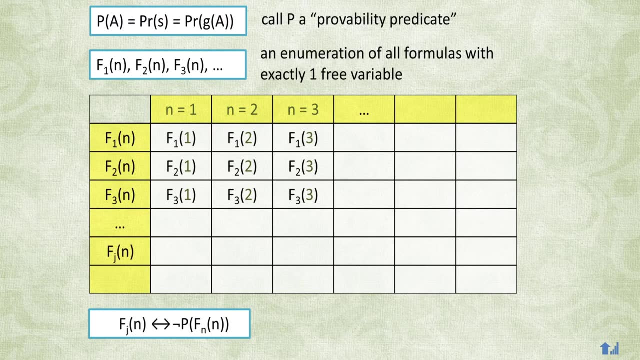 an output that is also a natural number. Nothing tricky here. Consider the formula, not p- of fn of n. It must be in the list above since it is a formula with one free variable. Let's suppose it's fj of n. So this would be the case for any n meaning. 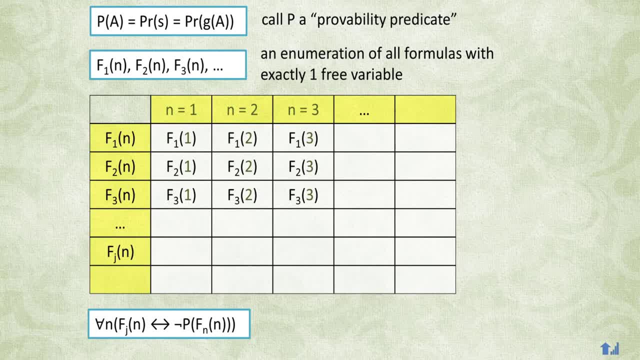 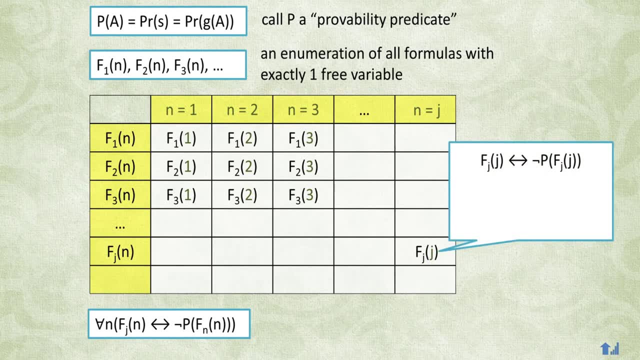 the function fj can accept any natural number. If we pick n equals j, then by diagonalization fj of j if, and only if, not p of n. To make the result clearer, we abbreviate: c equals fj of j. So the statement c implies that it's not provable. It is expressed as a theorem in. 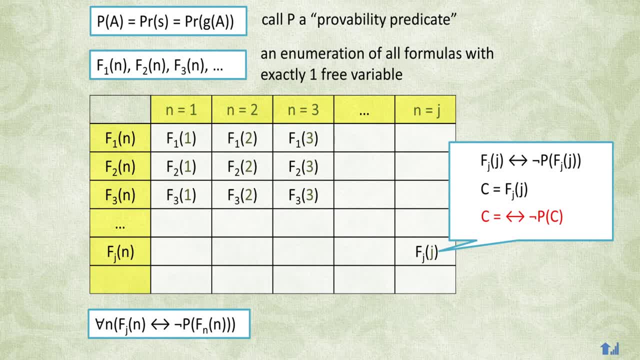 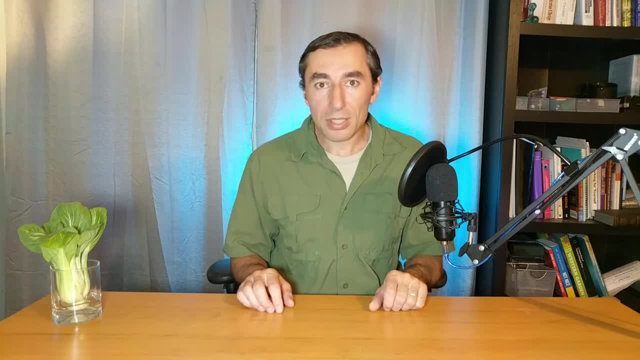 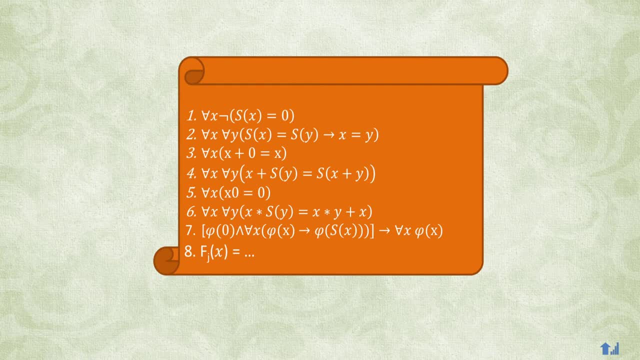 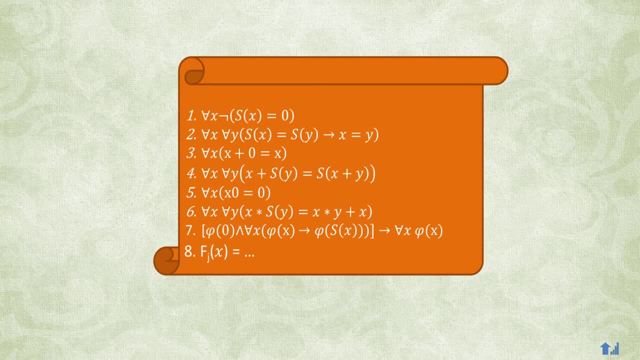 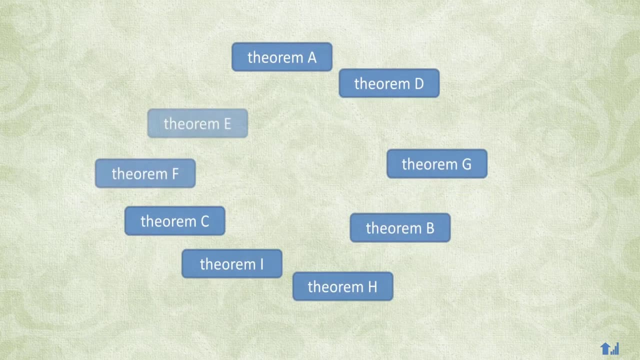 is not provable. If you think that all of this is rather inapplicable to other problems, remember that the self-reference may be done indirectly through a vast chain of intermediary links, In which case detecting such a self-reference means a similar algorithm. in itself, a certain sense can be adopted. 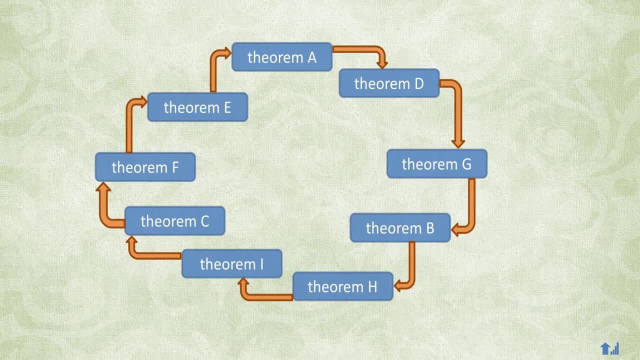 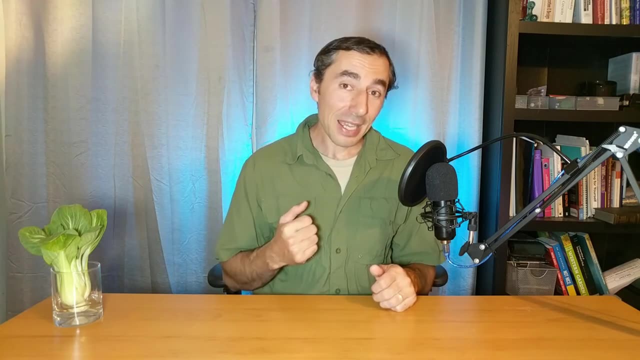 Even for case D, in which case this self-reference principle can just be defined as a proof. self-reference is not at all obvious. Since we've come so far, let me show you one more proof that's actually a little bit more intuitive. I'm not a mathematician, I'm a software engineer by training. 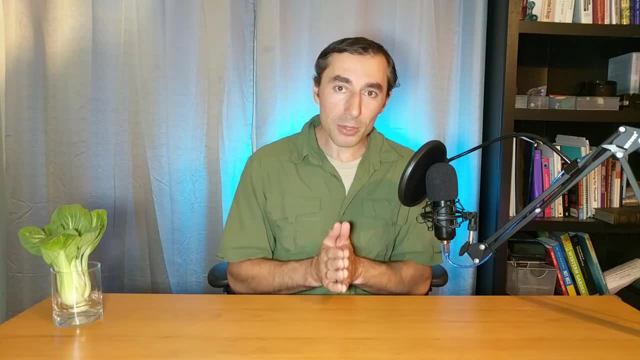 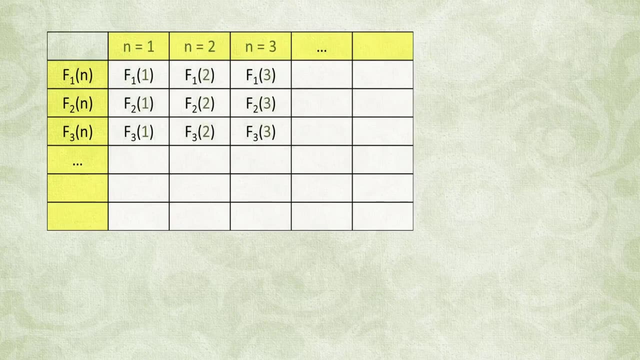 and if you are like me, you probably find the vocabulary that programmers use a little bit easier to digest. The concept behind this proof, however, is just as legitimate. The proof is based directly on Cantor's diagonalization argument, Just like before we create a list of all possible. 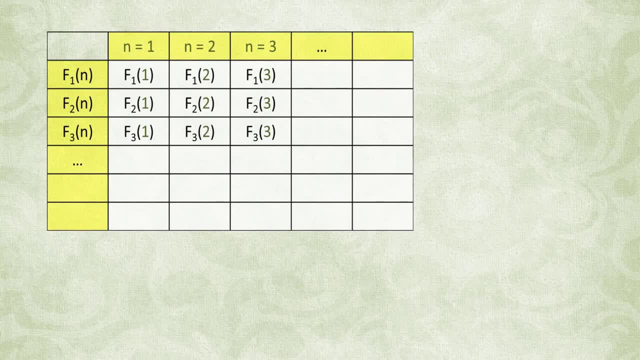 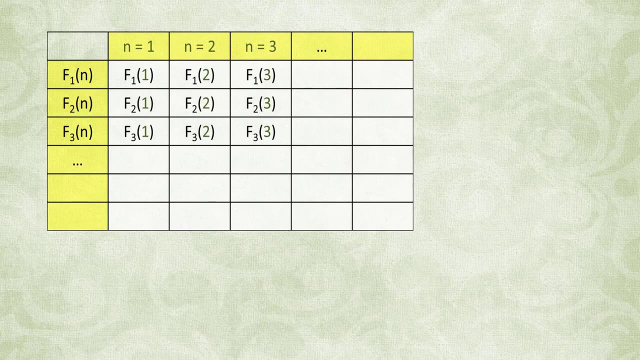 formulas with one free variable, Except now, we're going to call them functions instead of formulas that take in an integer parameter. Think of your favorite computer language, such as Java or Python as a context. There is an infinite number of these functions, but that's okay. There's an infinite. 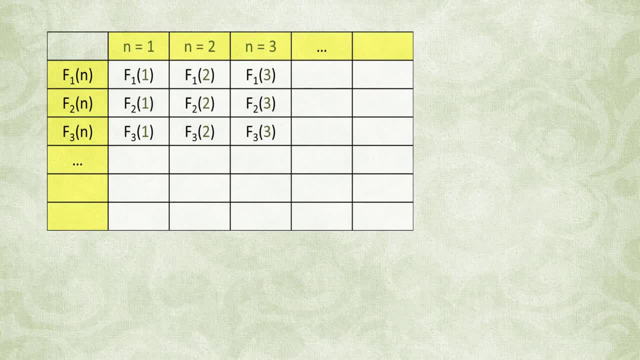 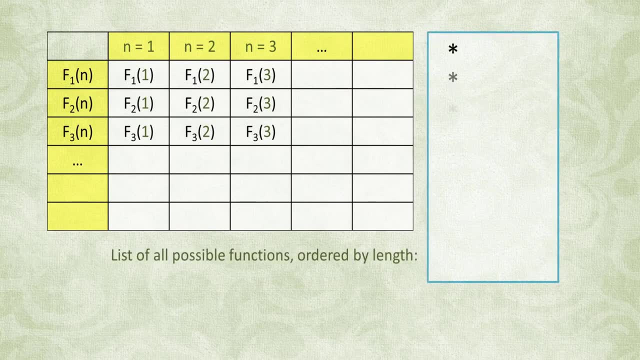 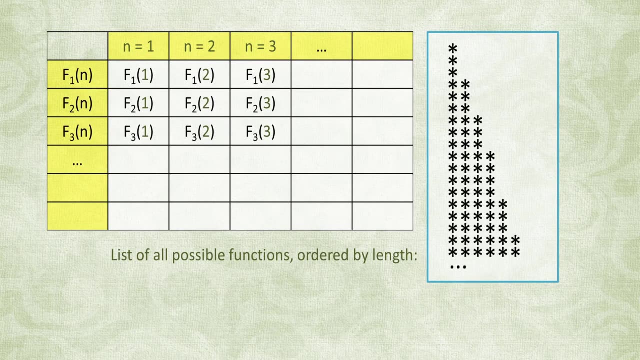 number of integers, yet we could still talk about them and do arithmetic with them. So how do we create this list? We can begin by writing a simple script that just goes through all possible combinations of characters. It first lists all possible strings of length 1,, then all possible strings of length 2,. 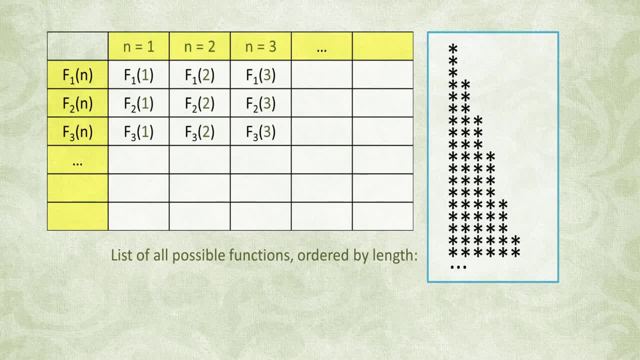 and so on. This is feasible since computer languages use a finite alphabet. Of course, not all combinations of characters are going to produce a function that compiles Those. we can just keep and not include in the list. We just care about the valid functions. 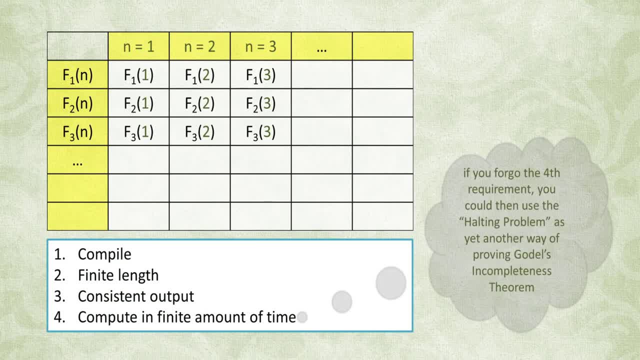 Valid, as in, just as what you'd expect, They compile. they themselves aren't infinitely linked. they consider each other as having two existing functions, and they don't weirdly sorta interact with one another. So we can call them functions and or them loops, And then we can take an integer function and compare them to each other. 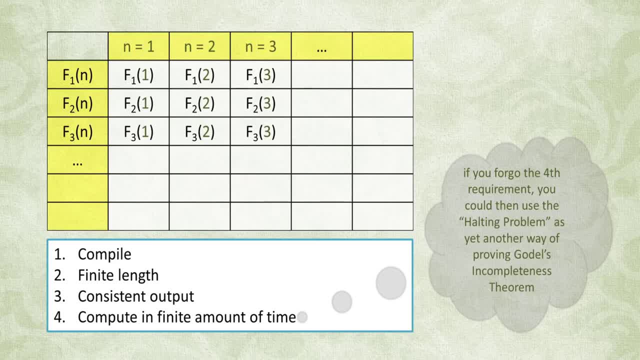 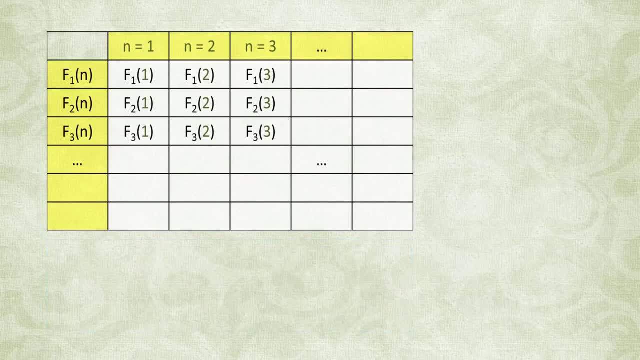 So we can take an integer function and or them loops. And then we can take an integer function, consistently produce the same output for a given input in a range of natural numbers, and the output is produced in a finite amount of time. Now we construct a special function. Let's call it q. 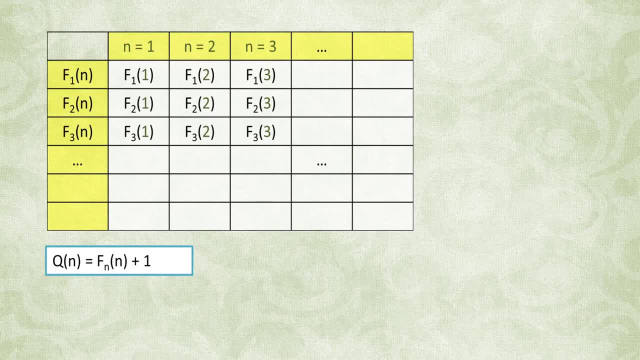 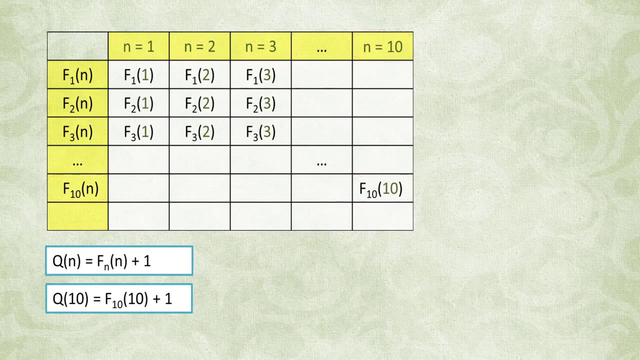 The way it works is that it takes its input parameter n and produces an output of the nth function in our list for the input n and adds 1 to it. For example, if the input parameter is 10, it produces whatever f10 would produce on. 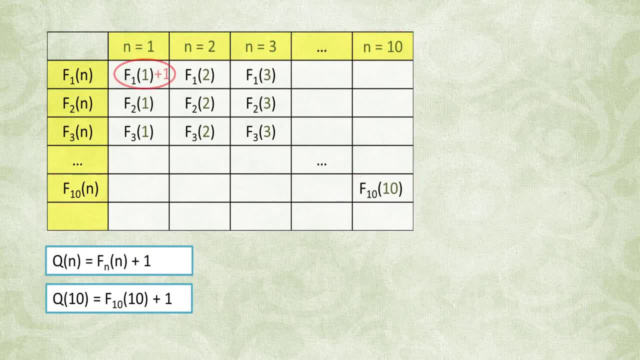 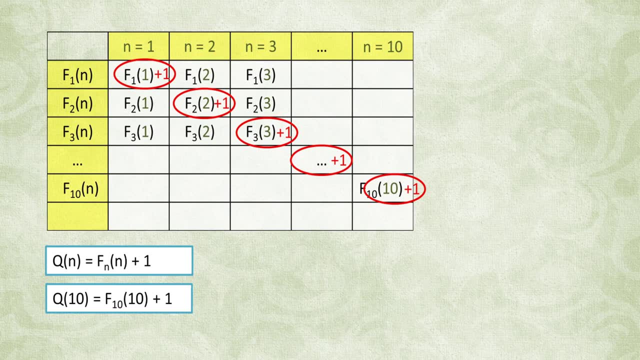 input 10, and then adds 1 to it. Since it does this for every integer, the output of this function could be read by just walking down the diagonal of our table and adding 1 to each value. The million-dollar question is then: is this function q in our list? 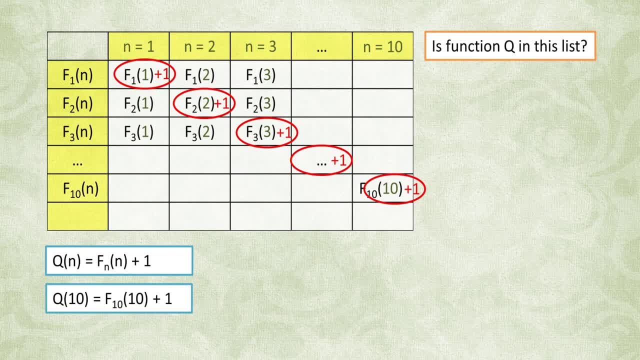 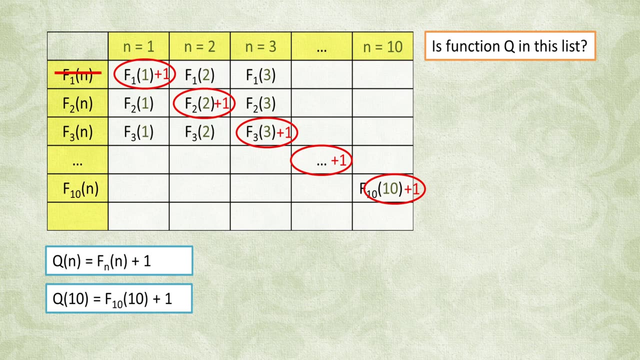 Originally we said that the list contains all possible single-parameter valid functions, But we know that q is not the first function f1, since it differs from it on input 1.. There may be other differences, but we know for sure that it differs at least on one input. 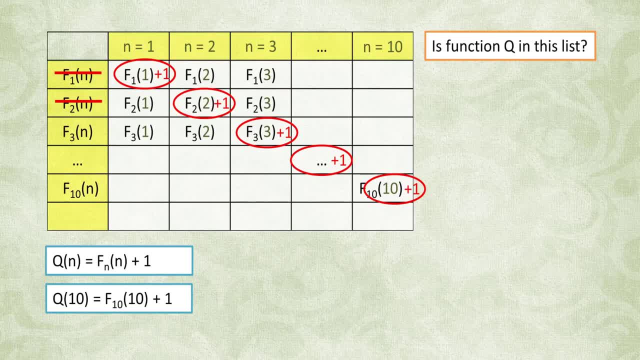 which is enough to say that it is different. We know that it's not f2, since it differs from f2 on input 2.. So this argument extends to any function in our list. In other words, q cannot be in this list. 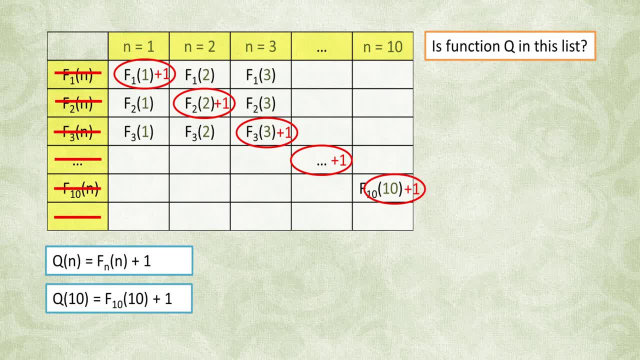 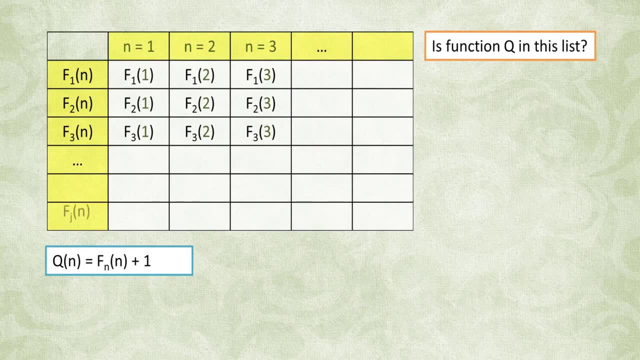 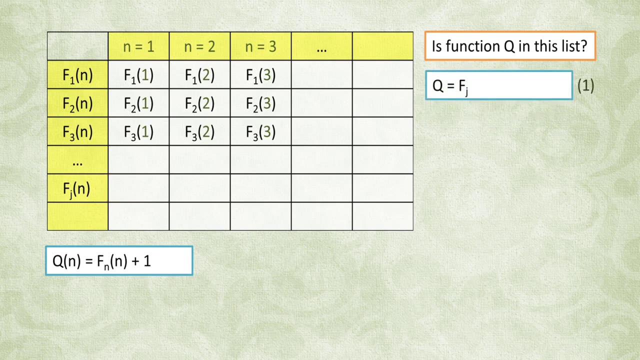 So let's see what happens. This is a contradiction to our original assumption that it's possible to list all valid functions, To state the same exact thing but from a different perspective, suppose it is in our list at some index j, So the function q is the same as function fj. 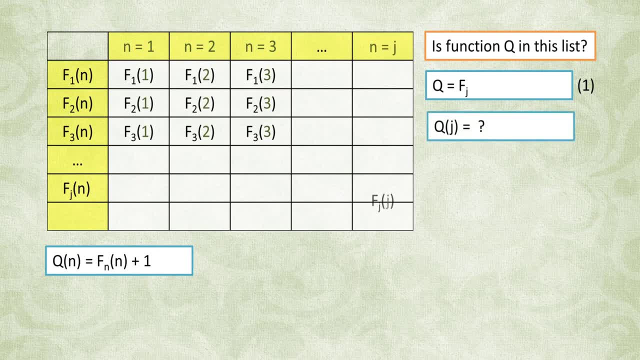 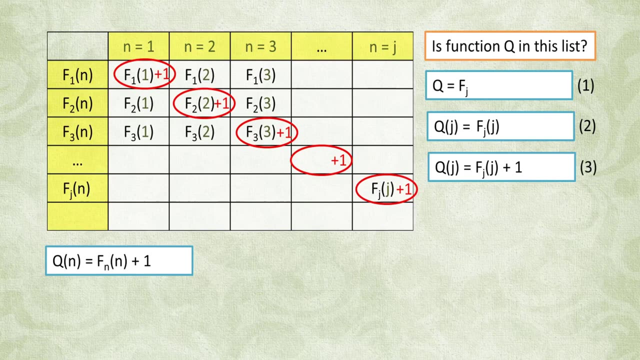 But then what value does it calculate for the input value of j? q of j would be fj of j, But by definition Function q is supposed to return the value on the diagonal plus 1.. So this is a contradiction, since number 2 and number 3 are clearly not the same. 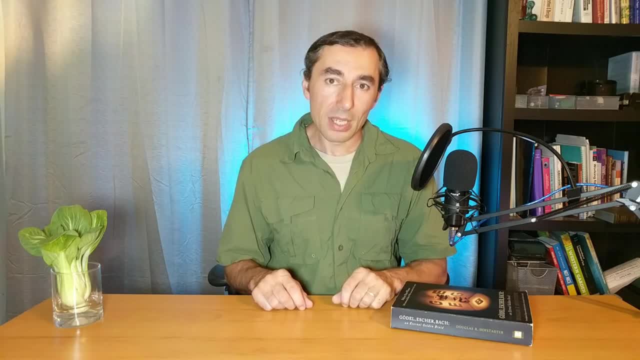 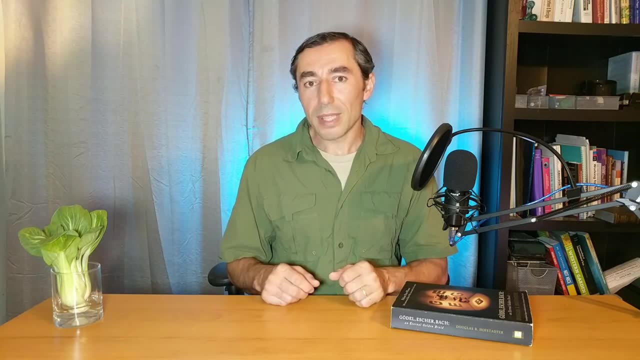 Shortly after publishing his first incompleteness theorem, Gerdelden published a second which states that any consistent axiomatic system cannot prove that the system itself is consistent. But that's something I'll leave for another episode. I hope you enjoyed this video. 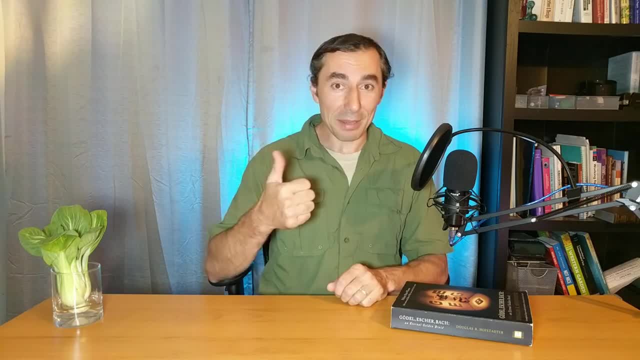 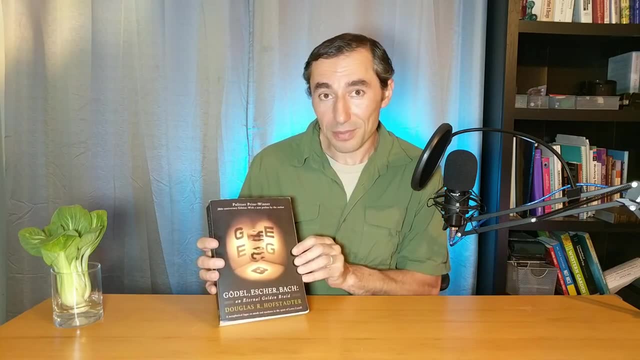 If you did. first of all, thank you. See you next time. If you liked this video, please do click that thumbs-up button. And secondly, I have a book recommendation for you. Gödel Escher Bach by Richard Hofstadter is full of mind-blowing ideas. 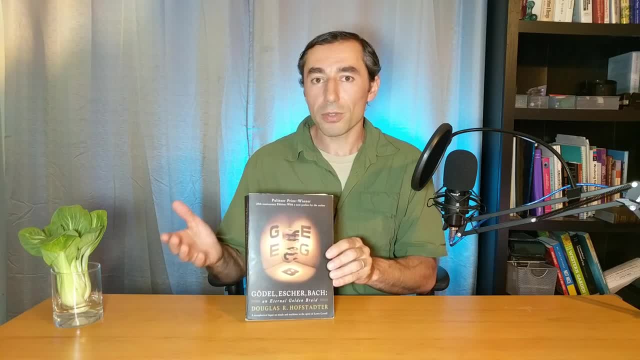 And they're presented in a way that doesn't require prior knowledge of computational theory or complex mathematics. Give it a read. I'm sure it'll give you lots to ponder about, And thank you for watching.